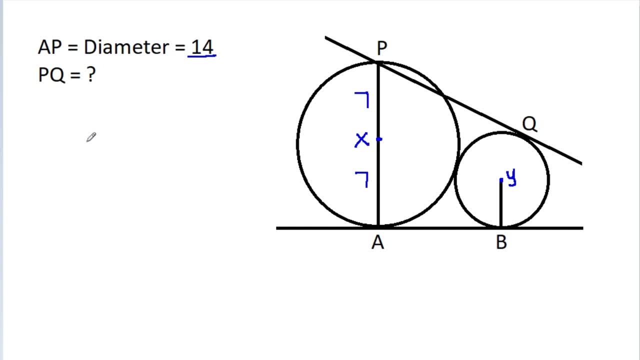 PX will be 7 and in any circle, radius and tangent are perpendicular to each other, So this angle will be 90 degree. this angle will be 90 degree And if we join Y cube, then this angle will be 90 degree. And now, if we join PY, then Y cube, this angle will 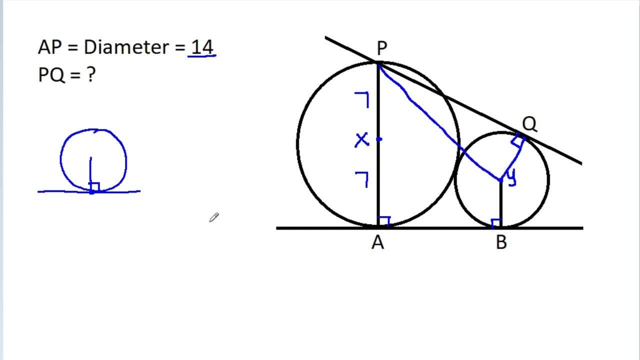 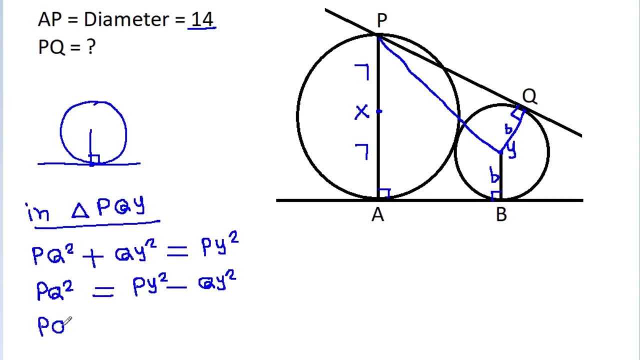 be 90 degree, Then in triangle PQY, PQ square plus QY square it will be equal to PY square and PQ square it will be equal to PY square minus QY square. And suppose radius of a smaller circle is B, then PQ square, it will be equal to PY. 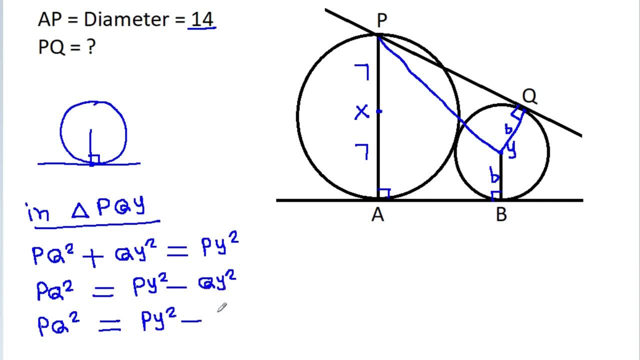 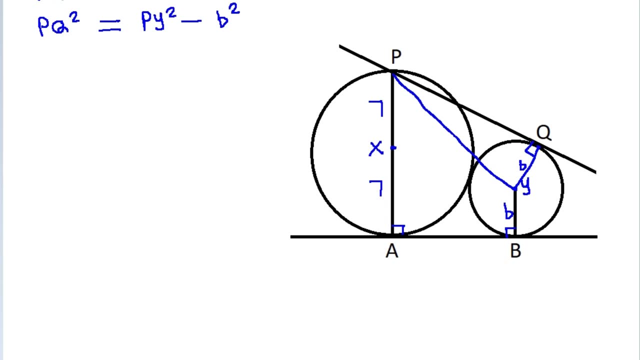 square minus QY square. Now, if we draw a perpendicular from Y on AP- suppose this point is M- then it will be ABYM, then in ABYM it is ABYM. this angle is 90 degree. this angle is 90 degree, this. 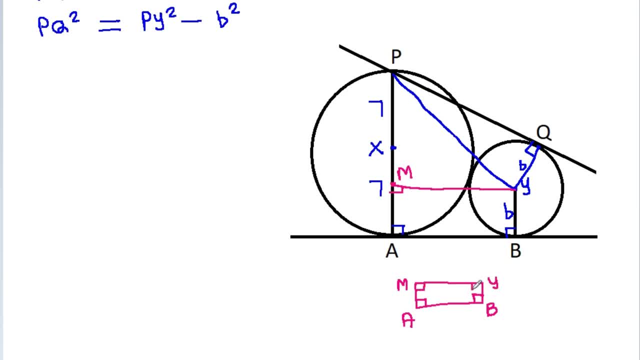 angle is 90 degree, so this angle will be also 90 degree, so it will be rectangle. And YB is B, so MA will be B, And we have AP is 14 and AM is B, So PM it will be equal to AP minus AM. 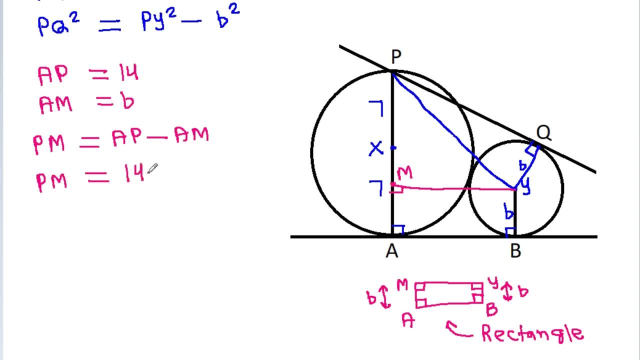 So PM, it will be equal to 14.. So PM, it will be equal to 14.. So PM, it will be equal to 14.. 14 minus b, Pm is 14 minus b, And also ab, it will be equal to my. So in triangle, Pmy. 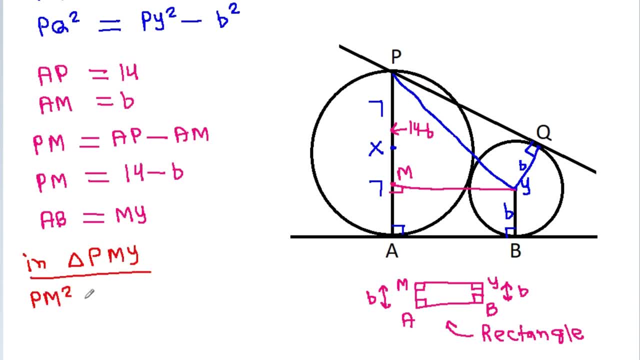 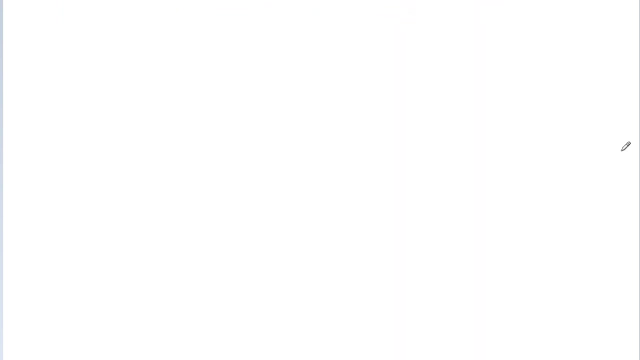 Pmsq plus mysq, it will be equal to Pysq, And Pm is 14 minus bsq. plus my is absq, It is equal to 14 minus bsq And from here Pysq, it will be Pqsq plus bsq. And if two circles are touching each other and they 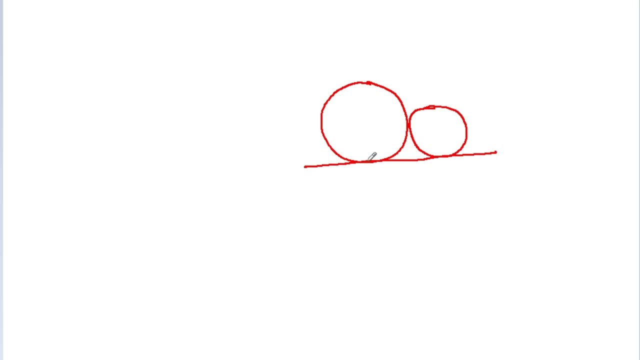 have a common tangent: it is a and b, And center is x and y. And suppose radius is a and b, Then if we draw a perpendicular from y on xa, suppose this point is m, Then if we draw a perpendicular from y on xy, it will be equal to: this is a, this is b, So it will be a plus b. 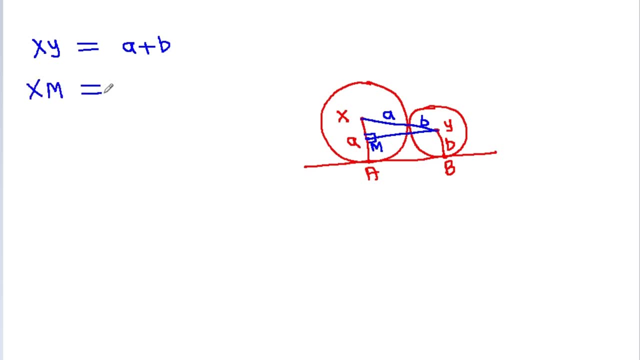 And Xm, it will be equal to Xa minus ma, And it is Xa minus ma is Yb. That will be a minus b. So in triangle x, m, y, x m square minus m- y square it will be equal to x y. 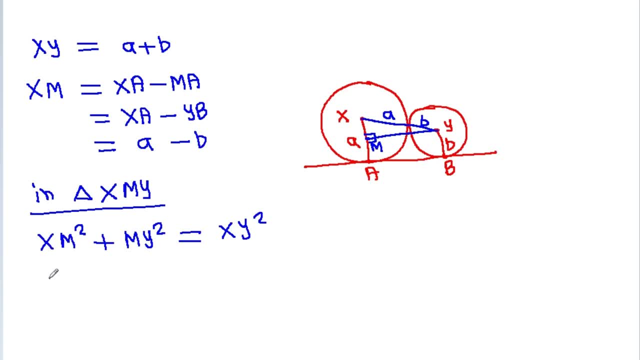 x square and x m is a minus b square, minus m y square. it is equal to x. y is a plus b square and it is a square plus b square minus 2ab plus m y square. 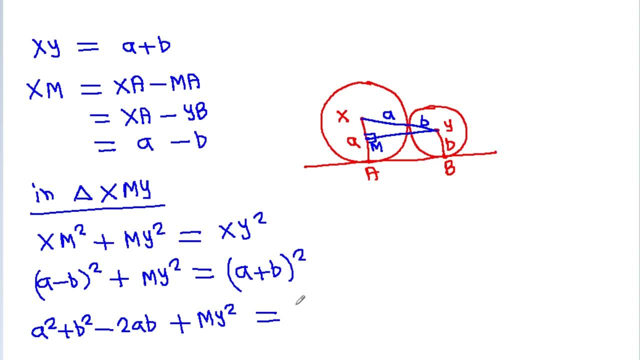 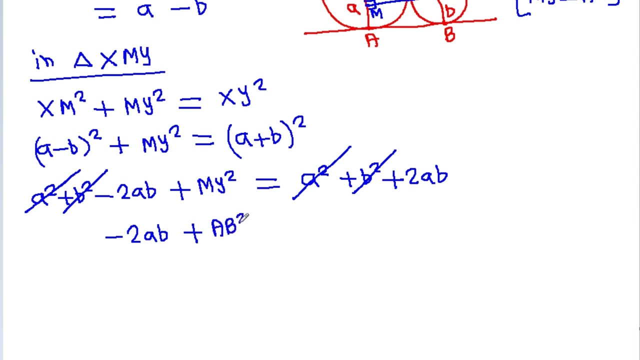 it is a equal to a plus b square is a square plus b square plus 2ab, and a square will get constant. b square will get constant and my it will be equal to a- b. so minus 2ab, minus a b square, it is equal to 2ab, so a b square will be equal to 4ab. 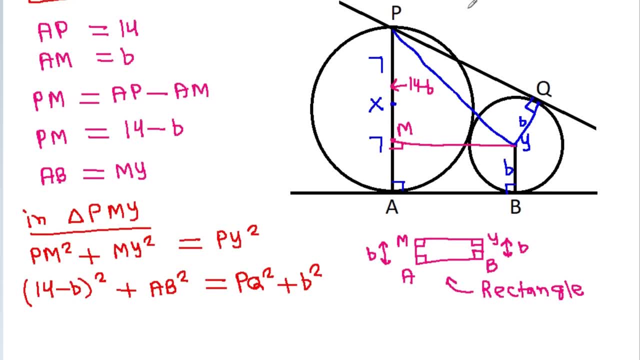 and here we have 14 minus b, a square plus and ab square, a b square, it is 4ab. and we have a is 7, so it will be 4 times 7 times b, that will be 28b. so it is 28b, that is equal to.